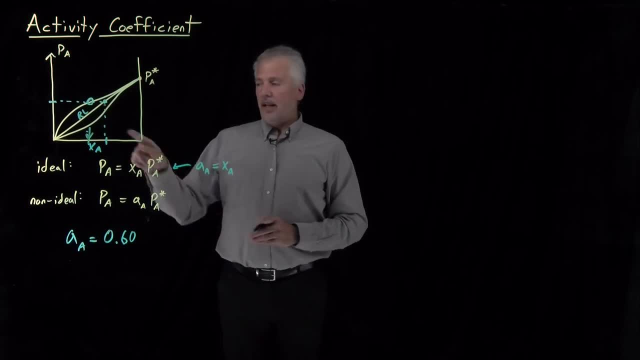 the same partial pressure of a at a mole fraction of 0.6.. And so, in terms of optimal value that works, is this a non-ideal solution, with the partial value of 0 point one partial pressure, as the ideal solution would have had at a mole fraction of 0.6,. 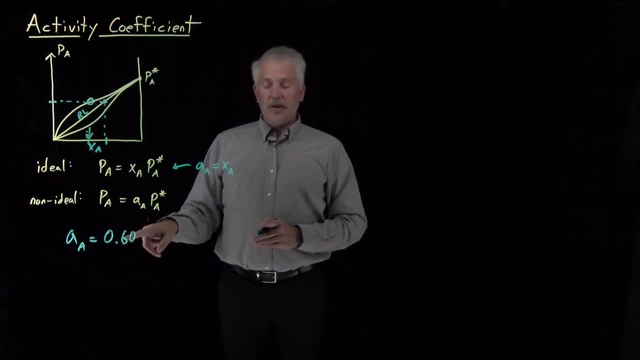 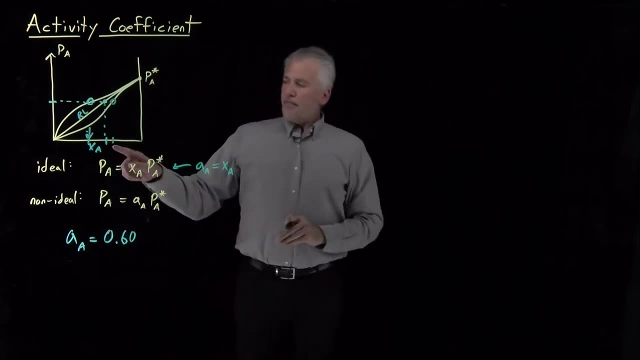 because the solvent A is more active in this solution than we'd have predicted just from Raoult's law. Likewise, if we have negative deviations, maybe we need a mole fraction of 0.65 or 0.7 to have this partial pressure. 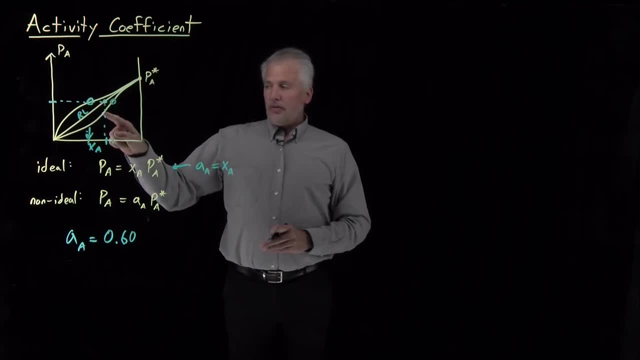 which is the same as the ideal Raoult's law solution would have had with a mole fraction of 0.6.. So that's what activity means. Often we'd rather intuitively just think about: okay, am I above or am I below? 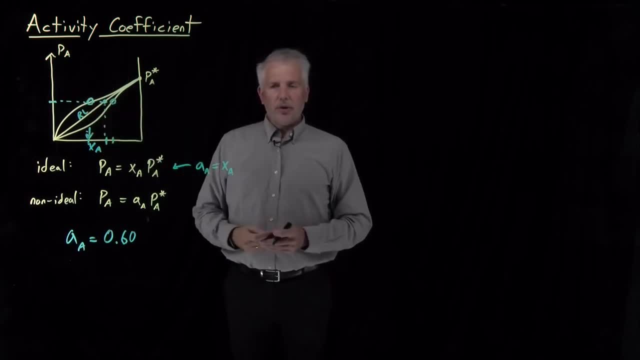 Am I exhibiting positive deviations or negative deviations? That's a more intuitive way to think about how the solution is behaving, rather than the mole fraction that the ideal solution would have had to have So often. what we talk about instead is not the activity, but the activity coefficient. 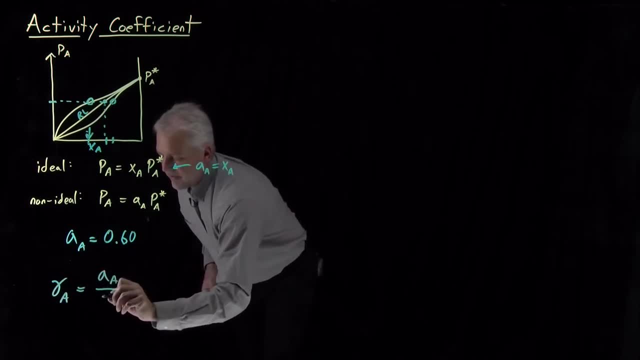 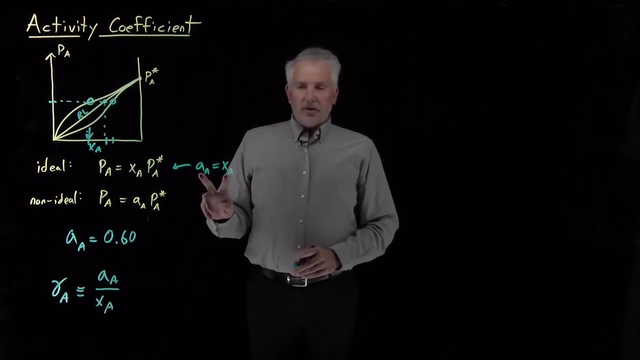 So if I take the activity divided by the mole fraction, so again I'm defining this quantity. Remember, in a perfectly ideal solution, the activity and the mole fraction are the same. The activity is the same as the mole fraction if the solution behaves ideally. 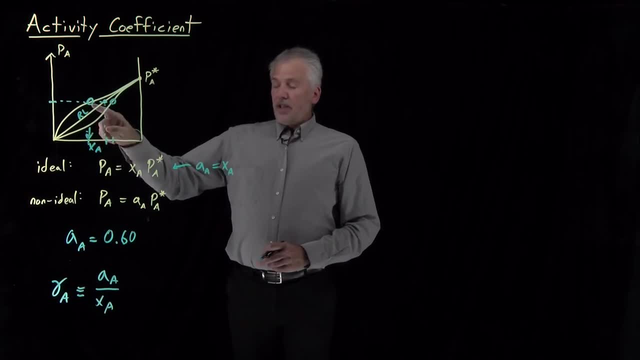 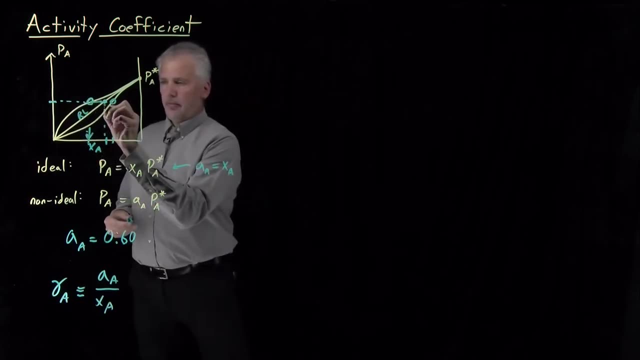 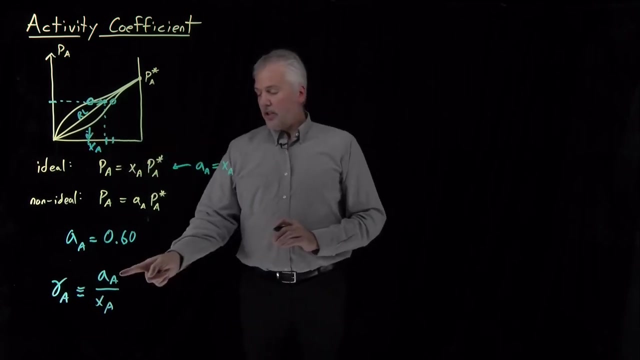 In a system with positive deviations, the activity's gonna be greater than the mole fraction. In a system with, because the partial pressure is greater than we'd expect, In a system with negative deviations, the activity is lower than the mole fraction, So I can use this ratio of the activity. 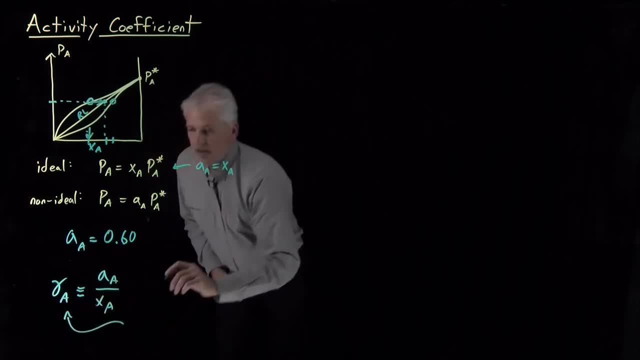 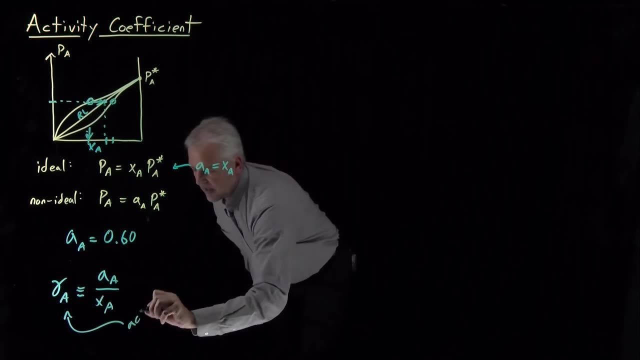 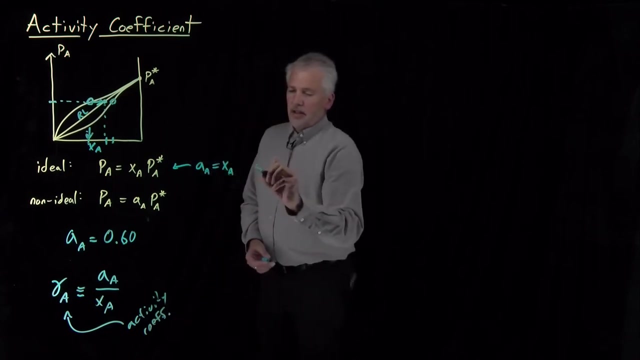 to the mole fraction to define how ideal the solution is That activity will be exactly equal. activity coefficient will be exactly equal to one in the ideal case. So that's the activity coefficient. In the ideal case, the activity coefficient is equal to one. 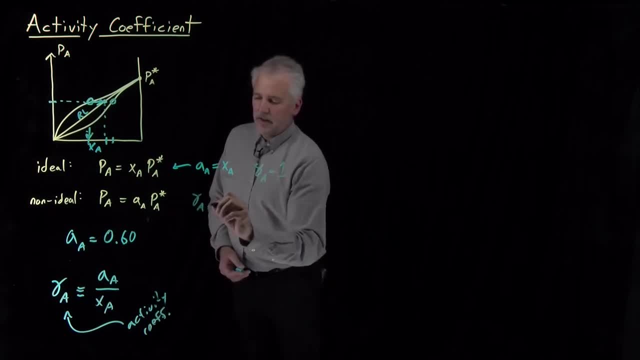 In the non-ideal case, the activity coefficient is less than one instances. population is less than one if we exhibit negative deviations, and then� negative deviations from Raoult's law, or the activity coefficient is bigger than one if we're exhibiting positive deviations from Raoult's law. 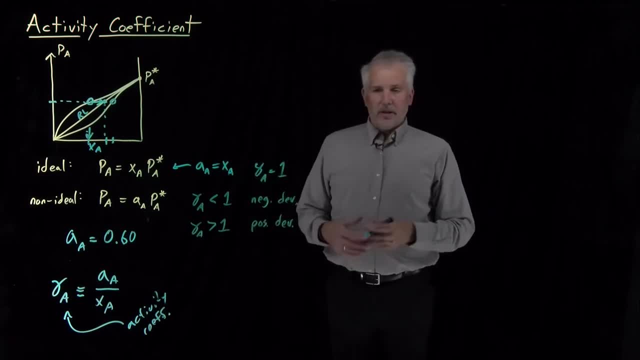 So that's usually an easier way to think about what's going on. If I tell you the activity coefficient is 1.1, then you know immediately the activity is 10% higher than it would have been if the solution's ideal. So that's usually a nice way to think about how non-ideal the solution is is to think: 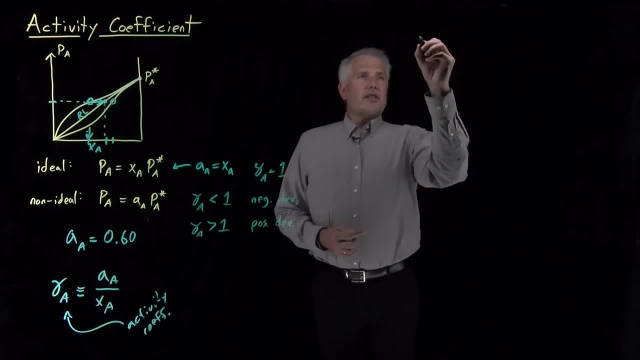 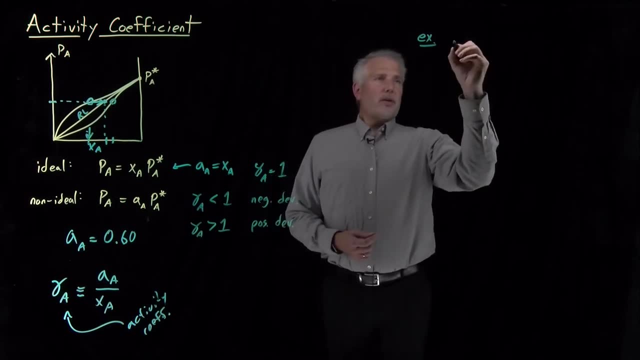 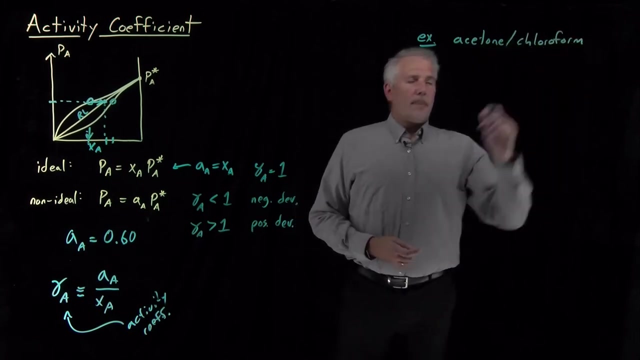 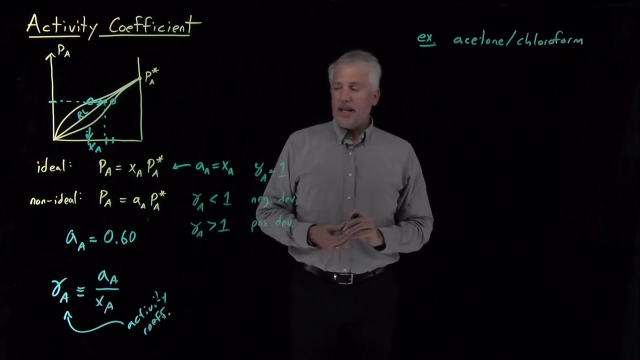 about the activity coefficient directly. So let's work an example to make sure these ideas are relatively clear. So let's say we have this system that we've used as an example before, a solution of acetone and chloroform. So that will exhibit negative deviations from ideality, from Raoult's law, because the hydrogen 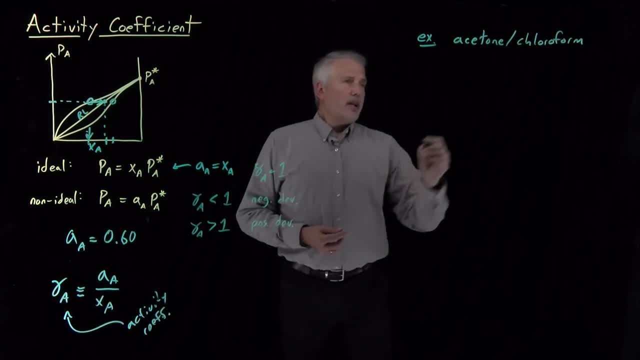 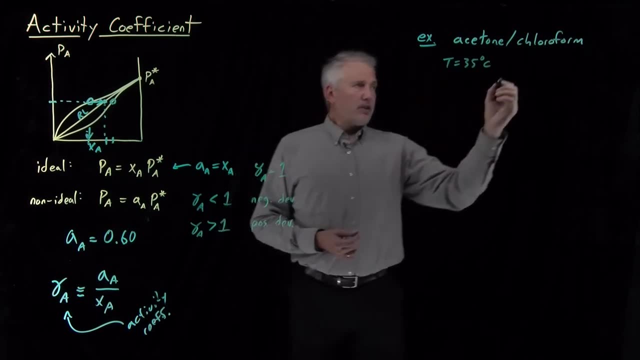 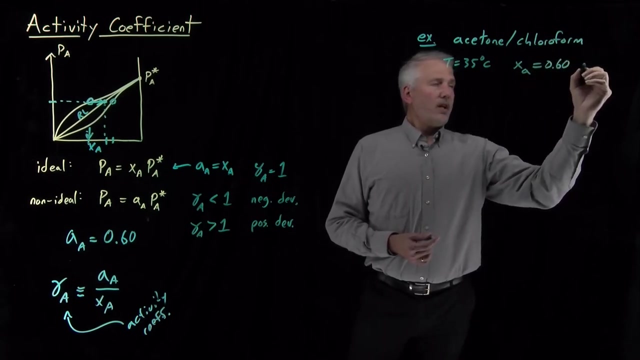 bonding between the acetone and the chloroform. Okay, And let's say we use some experimental data at if we prepare a solution, a 60-40 solution, so 60% mole fraction, acetone as a mole fraction, 40% chloroform. 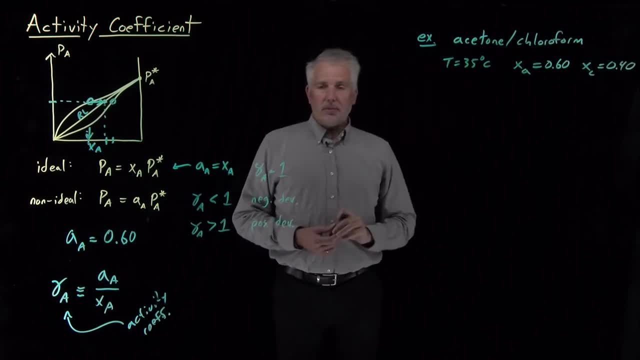 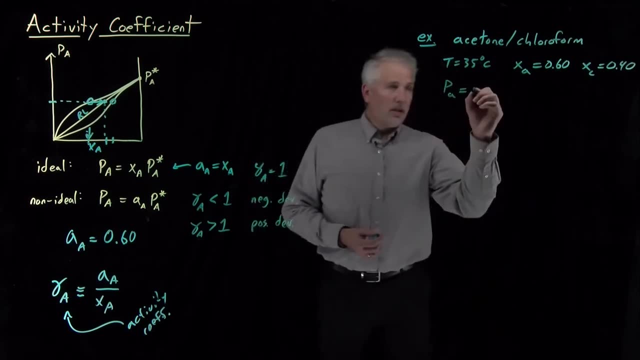 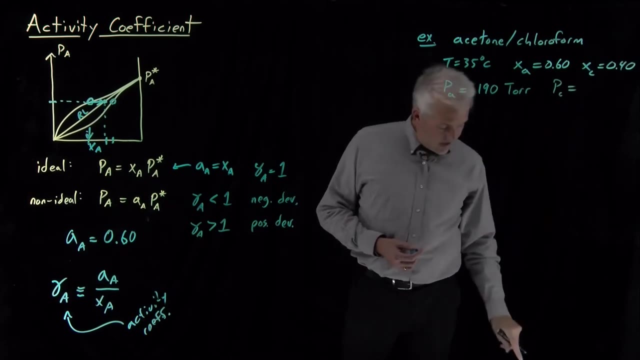 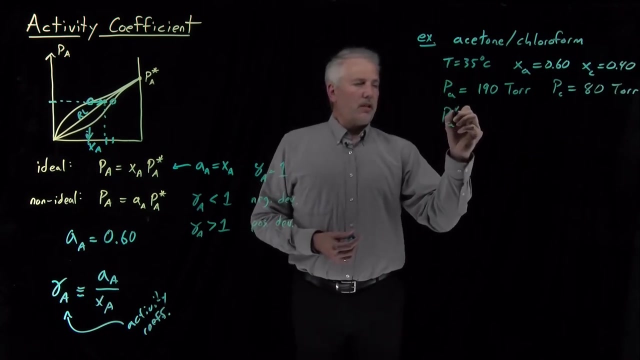 We can measure the partial pressures of the two substances above that solution. The partial pressure of acetone at 35 degrees Celsius will be 190 Torr. Partial pressure of chloroform will be 80 Torr And those can be compared to the vapor pressures for pure acetone as a solvent. 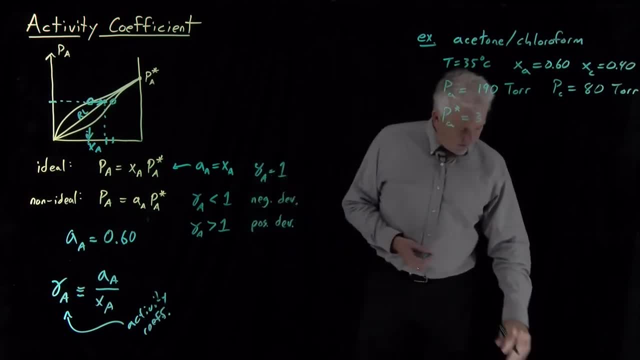 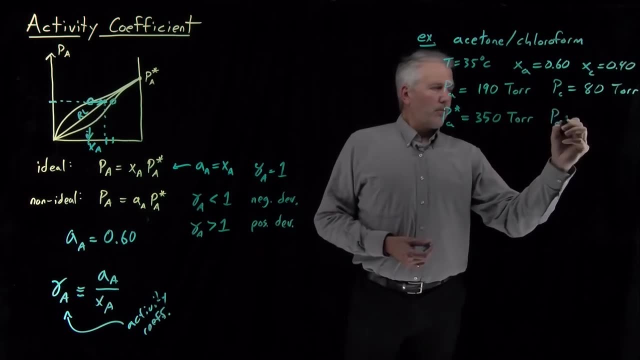 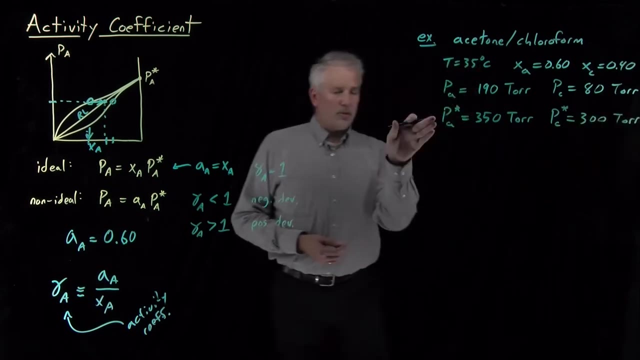 Pure acetone has a vapor pressure of 350 Torr At this temperature. Chloroform, At a temperature of 35 Celsius, has a vapor pressure of 300 Torr. So those two numbers we can look up, We can certainly measure them. 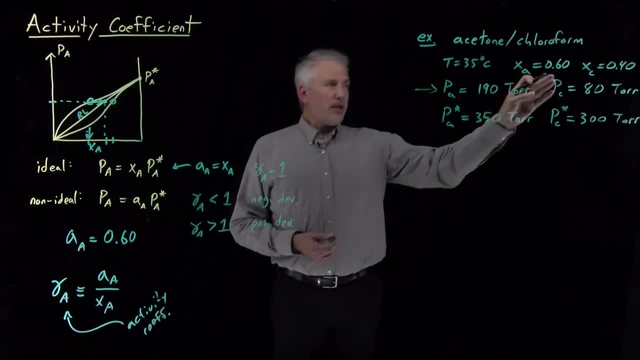 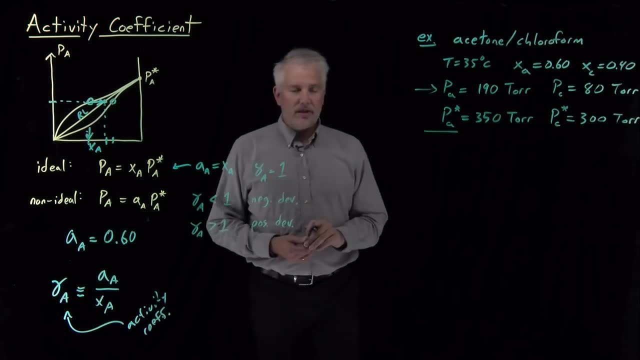 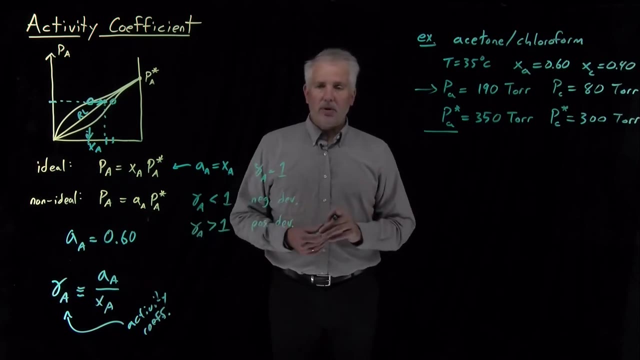 Of course, these partial pressures measured at 35 degrees Celsius are particular to that particular preparation of a solution. The question then is what are the activities of the two different solvents in this solution And what are their activity coefficients, And how do we interpret those values? 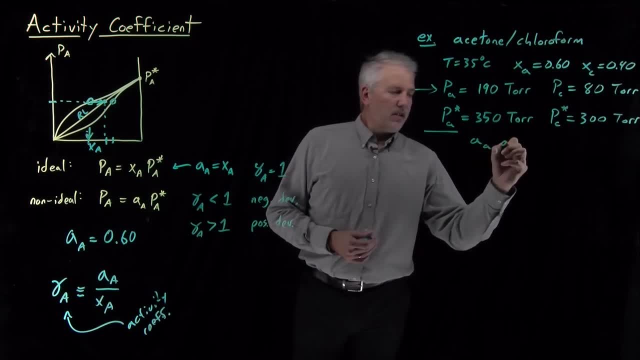 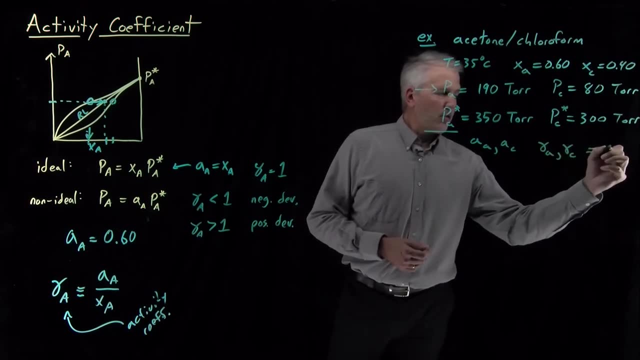 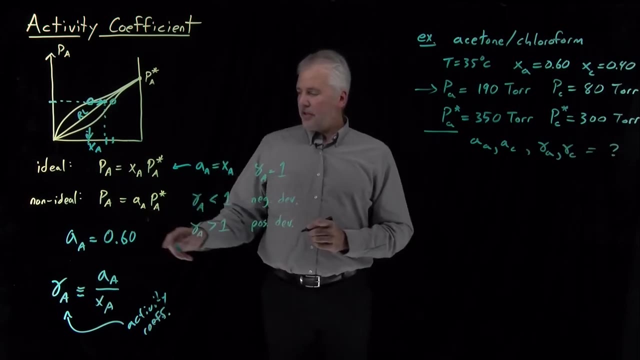 So Activities of acetone and chloroform, Activity coefficients of acetone and chloroform. What are those four values, So we can use our various definitions to obtain those. The activity is the ratio of a partial pressure to a vapor pressure. 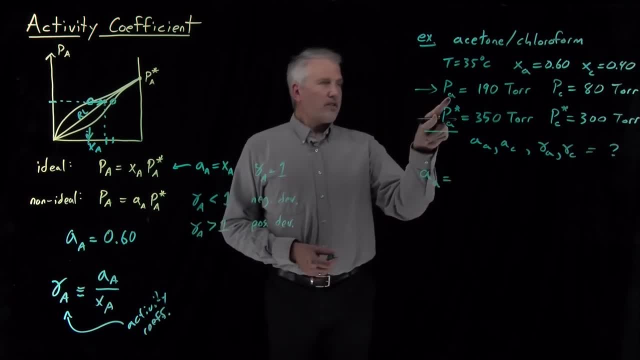 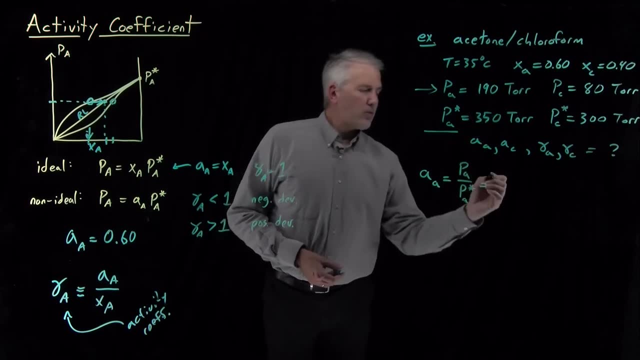 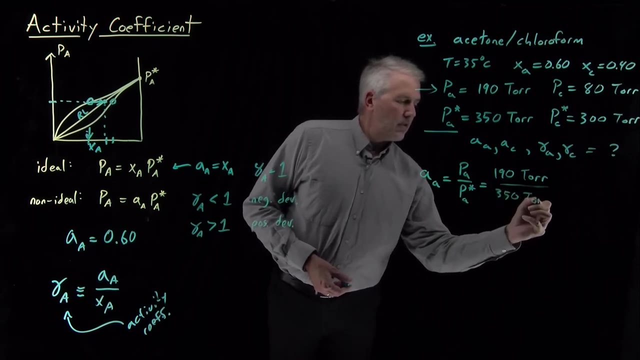 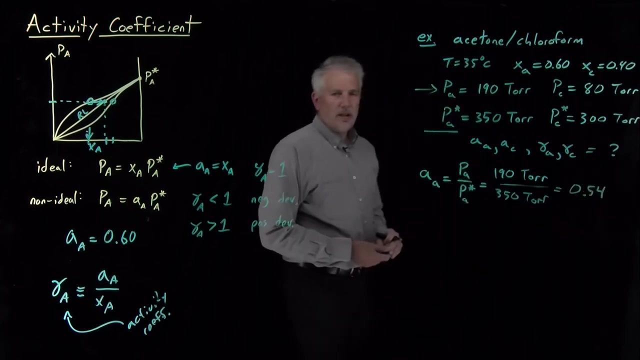 So the activity of acetone is its partial pressure, Okay. And then the activity of acetone over its vapor pressure. In this case, that's 190 Torr Over 350.. Which works out to be .54.. Okay, So there's a numerical result. 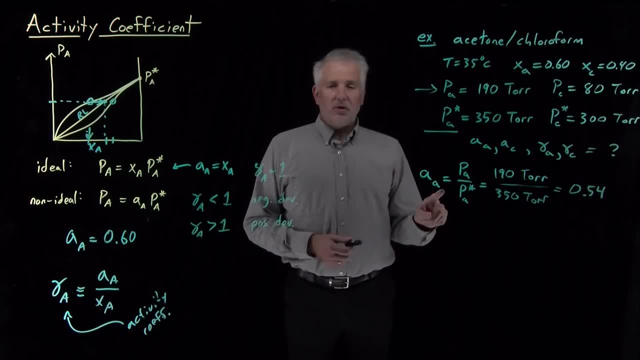 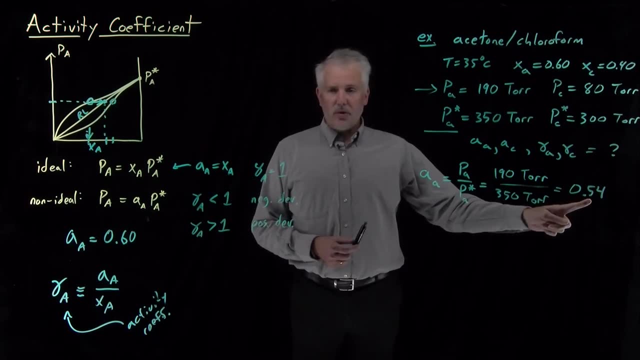 The activity of acetone is .54 in this solution. What does that mean? How do we interpret that number? Remember, Activity just tells us. This solution is behaving as if It had a mole fraction of .54 in this solution, 0.54. acetone, behaving like an ideal solution, would behave if its mole fraction was 0.54.. 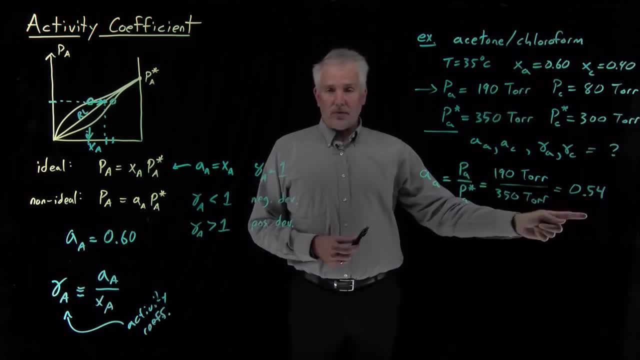 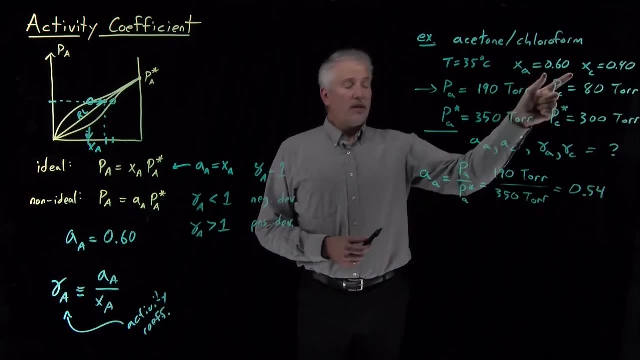 Its mole fraction is actually 0.6, not 0.54.. So that number is lower than this number. the solution is less. the acetone is less active than we would expect for a solution with mole fraction 0.6.. 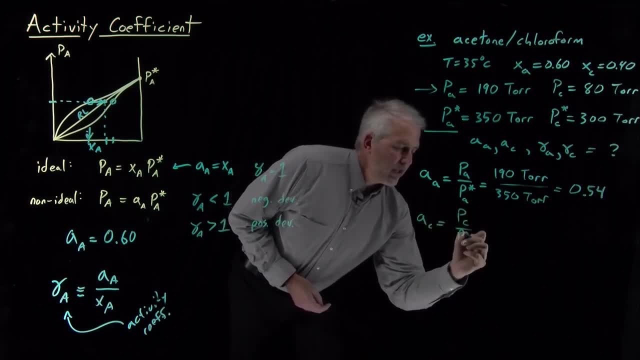 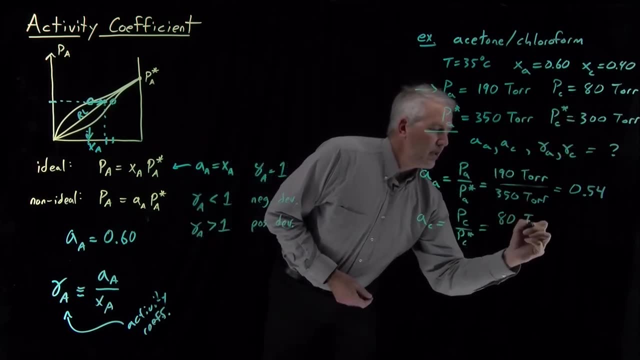 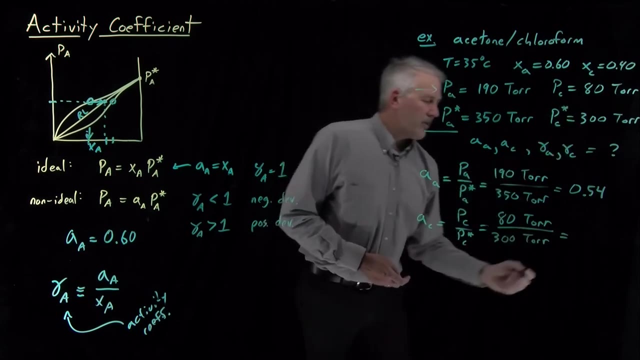 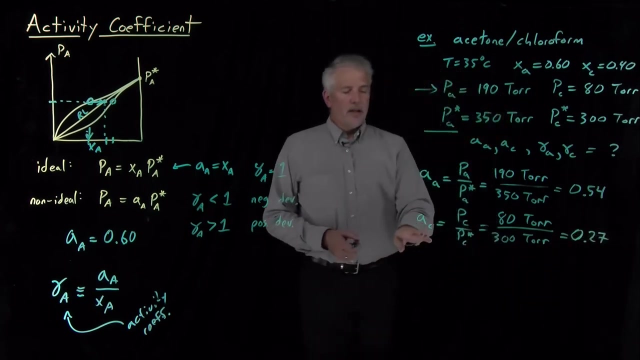 Likewise for chloroform. we can take the ratio of partial pressure to vapor pressure. partial pressure of 80, vapor pressure of 300. So 80 divided by 300, that gives us 0.27.. So again this solution, the chloroform in the solution, behaves as if it were in an ideal. 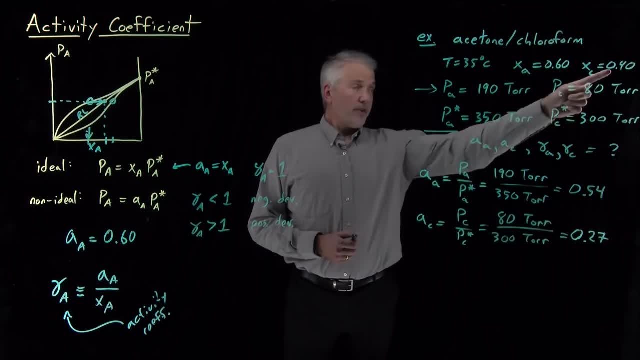 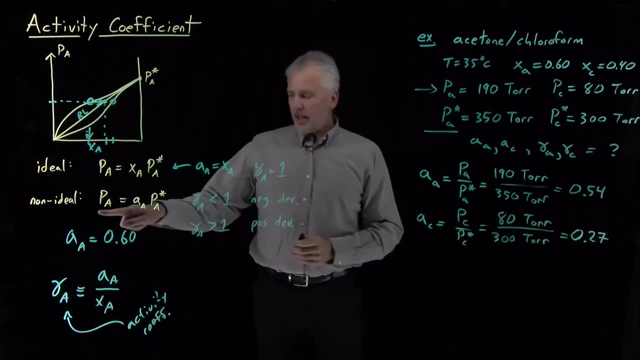 solution with mole fraction 0.27.. It actually has mole fraction 0.4,, but if we want to continue using Raoult's law, we have to pretend that it has 0.25.. A mole fraction of 0.27, that's what this equation is. 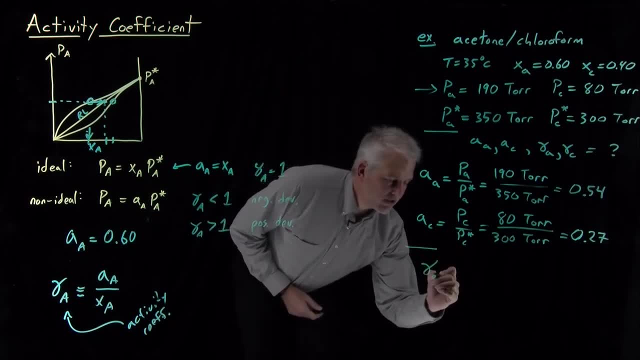 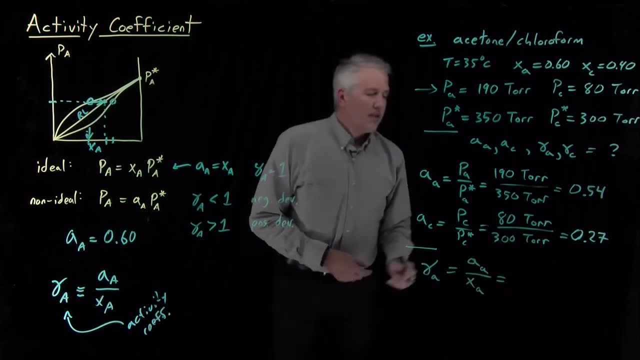 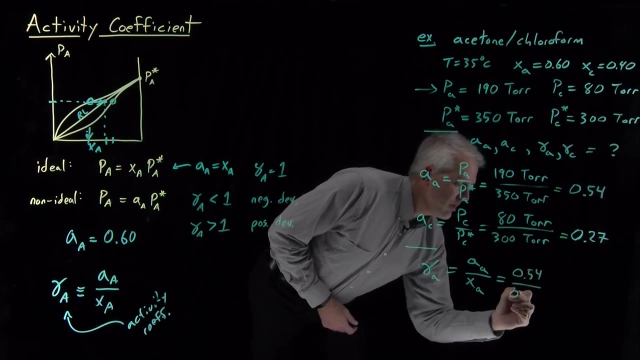 Now that we have those activities, we can calculate the activity coefficients. Activity coefficient of acetone being its activity divided by its mole fraction. Activity of 0.54 divided by a mole fraction of 0.6.. So 0.54 is 90% of 0.6.. 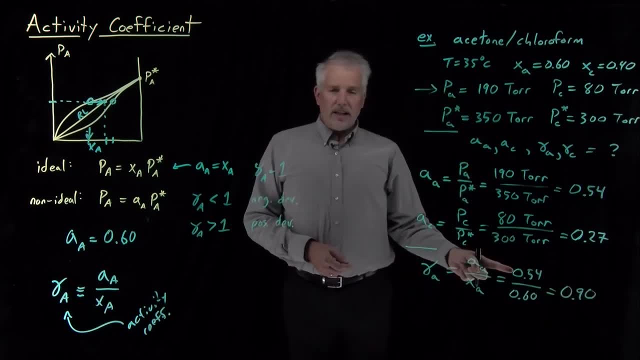 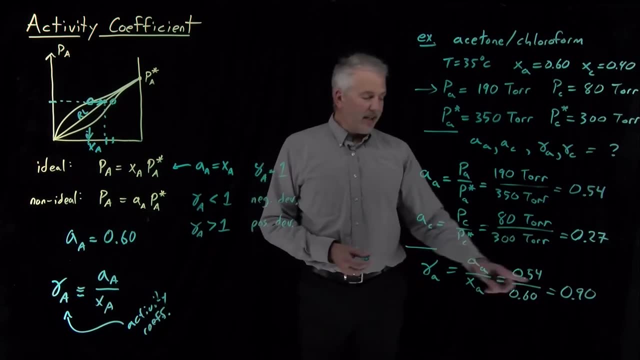 So that's the number that tells us. Acetone is only 90% as active as it would be in an ideal solution. So the activity coefficient is 0.9.. It's only 0.9 as active. So now we know, confirming what we expected would be true about acetone and chloroform. 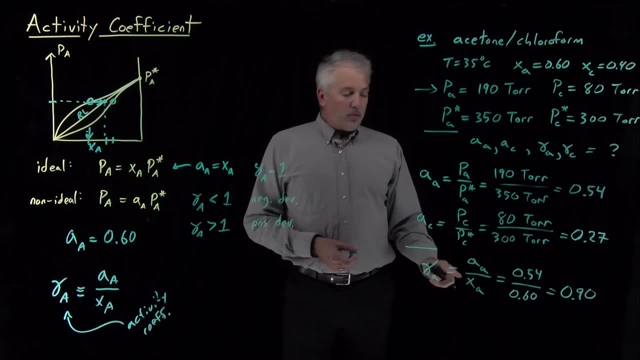 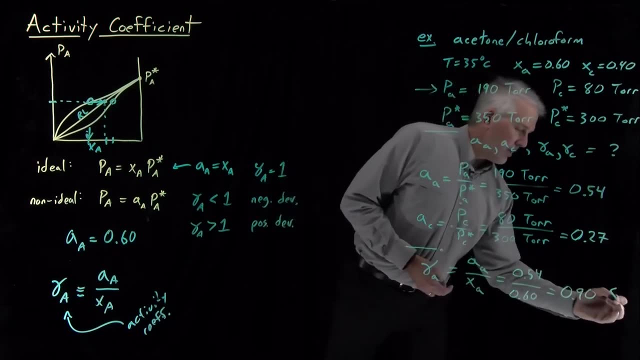 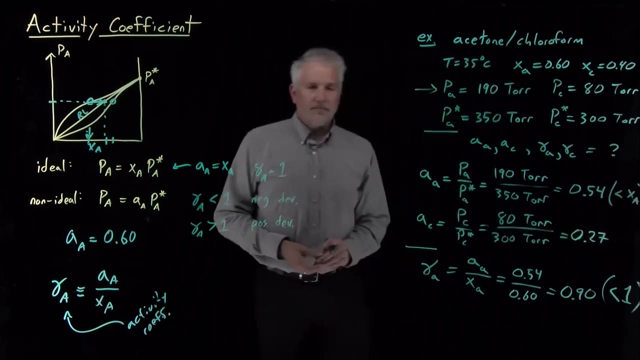 that this is a system that exhibits negative deviations from Raoult's law. The partial pressure is lower than Raoult's law would predict. The activity coefficient is less than 1, which means the same thing as saying the activity is less than the mole fraction. 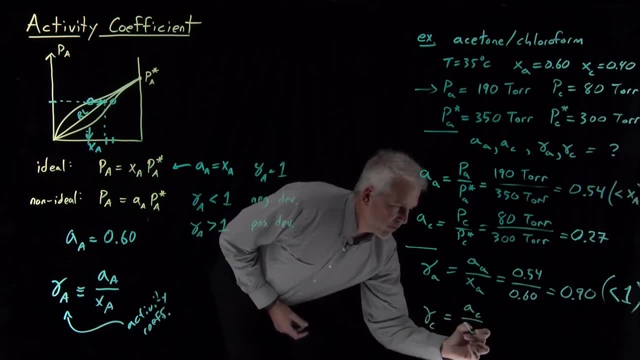 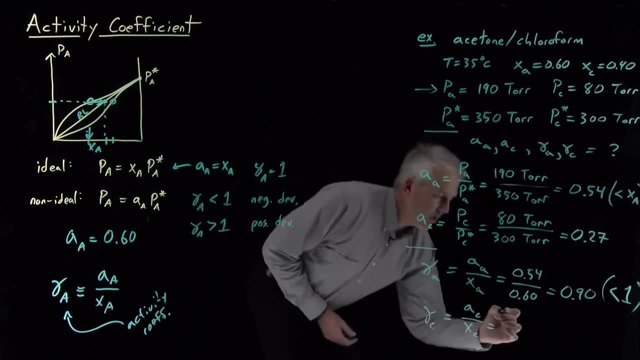 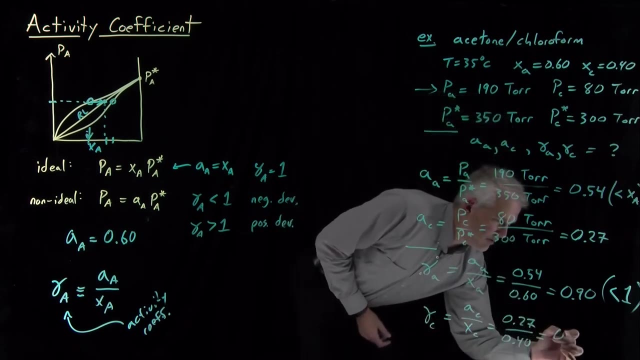 Similarly for chloroform. if I take the activity of chloroform over its mole fraction- activity of 0.27 divided by the mole fraction of 0.4, that is 2 thirds- Again, that value is less than 1.0.. 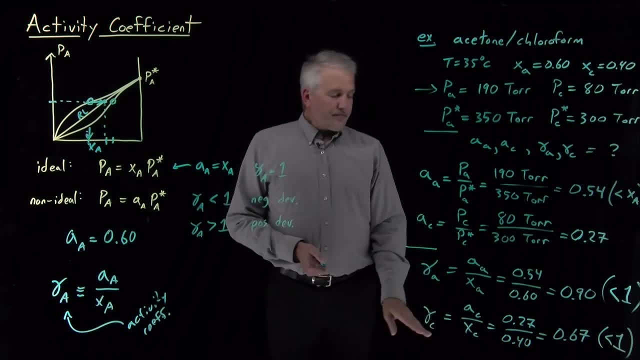 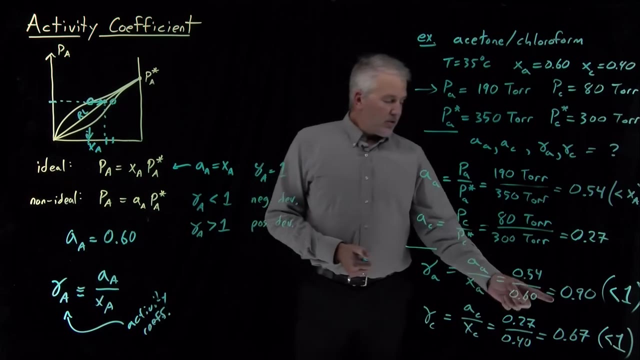 meaning that chloroform is also less active than Raoult's law would predict. in this solution It's exhibiting negative deviations from ideality. So both of these solvents have their partial pressures depressed by the existence of the other one. Notice that these two numbers are not equal. 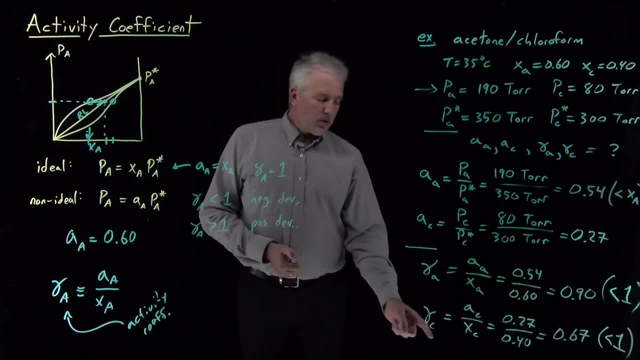 There's no reason they should be equal. What this means is that chloroform is more non-ideal in this case than acetone is. Chloroform has its partial pressure reduced more by the presence of acetone than acetone has its reduced by chloroform. 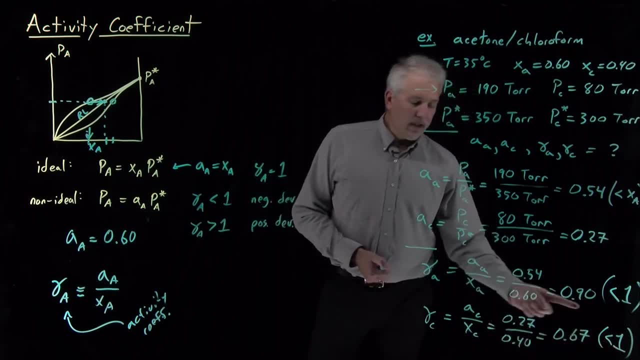 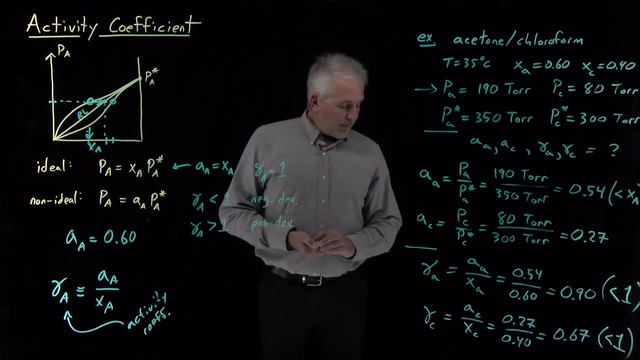 The deviation from the ideal case is larger for chloroform than acetone. Acetone has a stronger effect on chloroform than chloroform has on acetone. Okay, so that's a summary of the activity coefficient, which, as I've said, is maybe a more intuitive way to think about how a solution is behaving non-ideally. 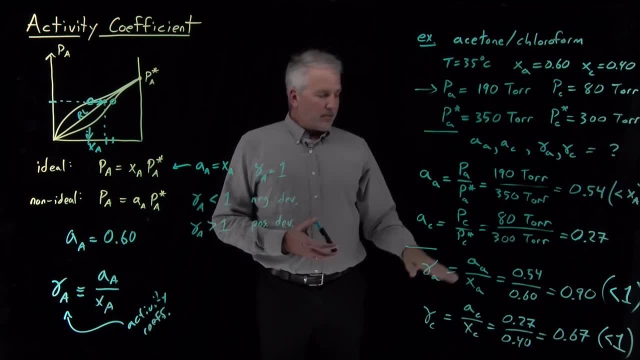 how non-ideal it is, as well as some examples of the relatively simple arithmetic that we use to determine acetylchloroform Activities and activity coefficients.